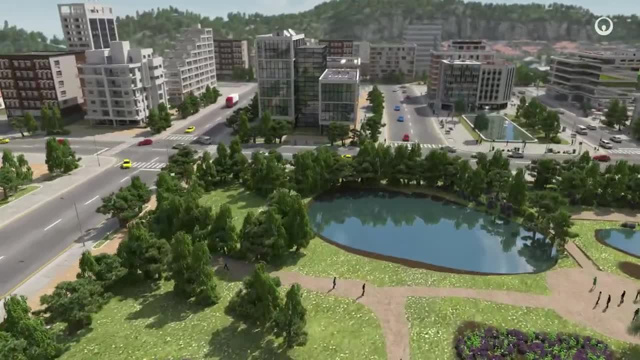 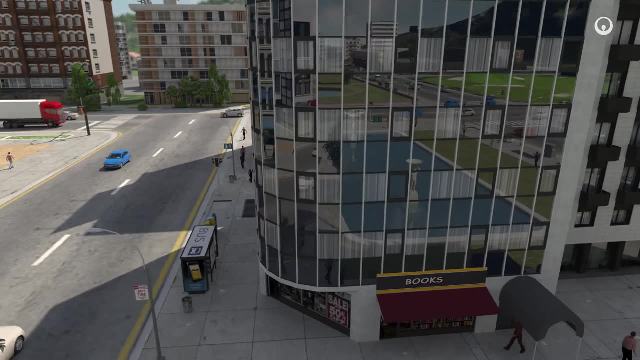 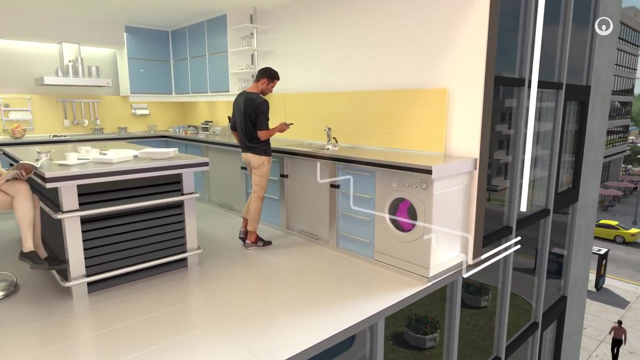 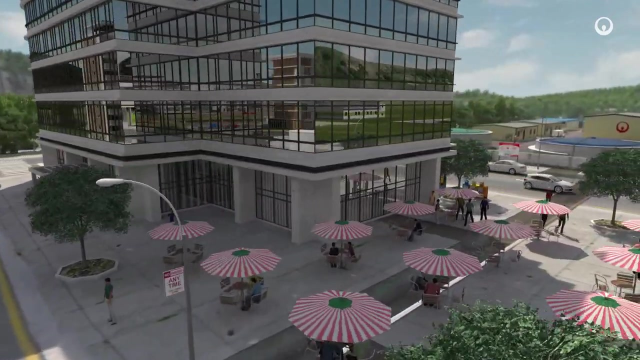 Locally recycling a portion of the wastewater helps protect water resources and reduces the environmental impact. Wastewater can come from factories and homes or from rainfall. Local sewer systems carry wastewater to the nearest treatment plant. A combination of treatment systems may be used, depending on the quality requirements for the treated water. 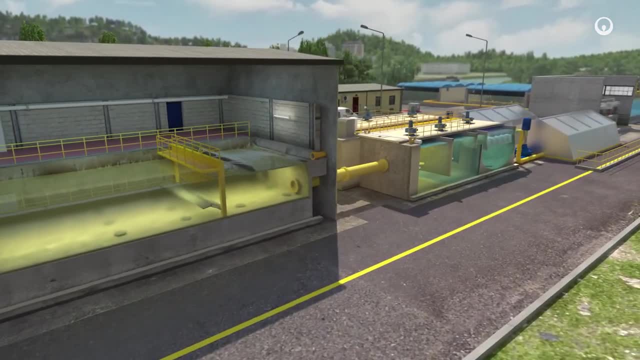 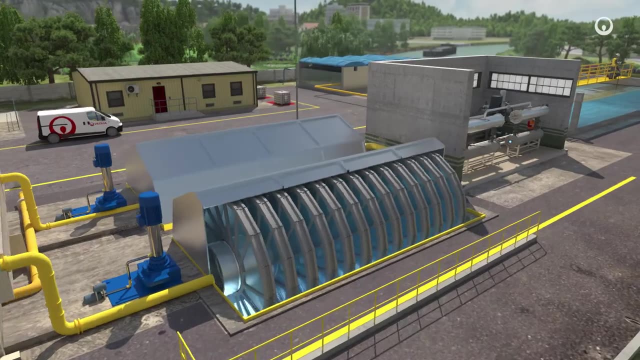 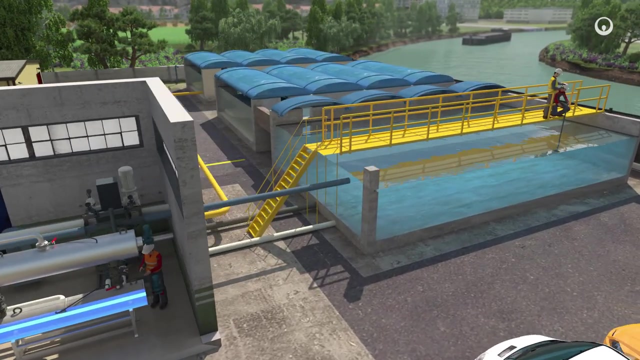 Settling tanks and biological treatments remove organic and mineral pollution from the water. Fine membrane filtration may also be used in combination with physicochemical disinfection to remove microbiological pollution. The treated wastewater meets all the regulatory, environmental and health requirements, depending on each particular type of use. 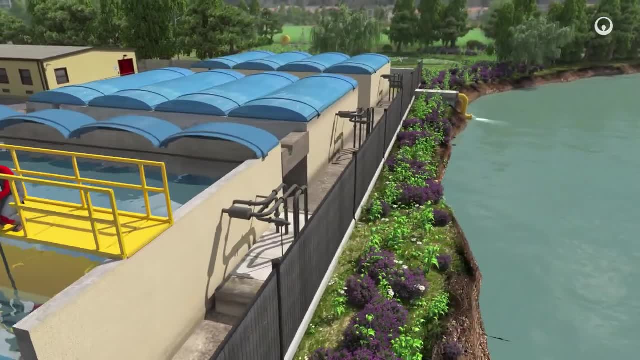 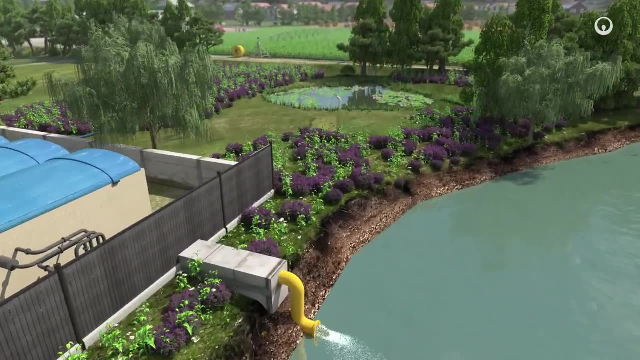 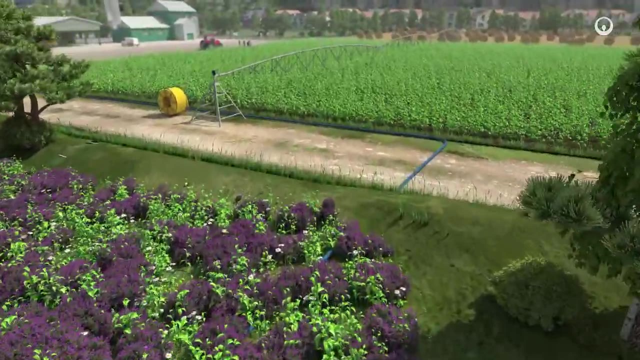 It is totally safe to reuse. Clean water can be simply released back into the natural environment. This helps to replenish water resources flowing into streams and rivers into water tables or wetlands. In agriculture, reusing treated wastewater for crop irrigation helps to secure harvests. 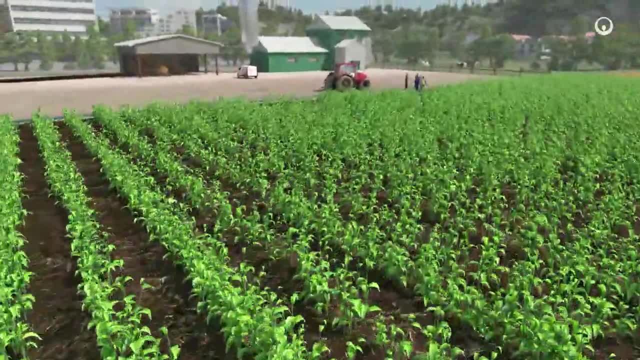 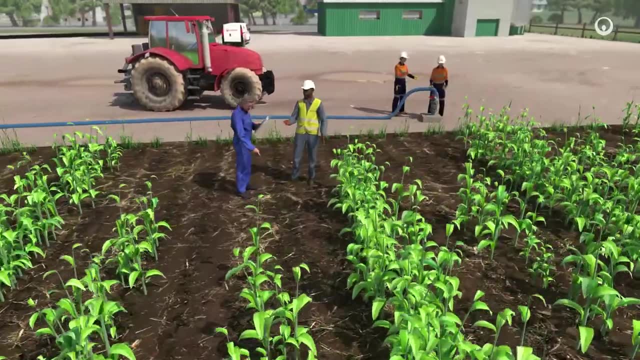 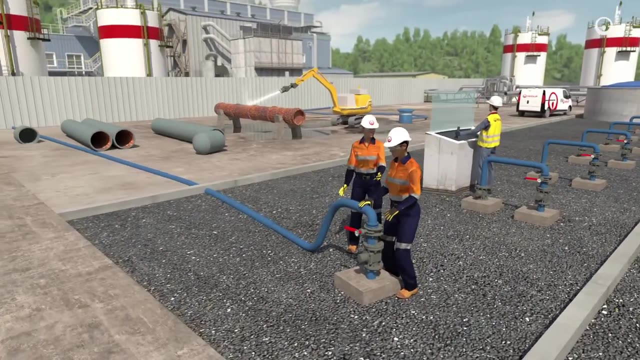 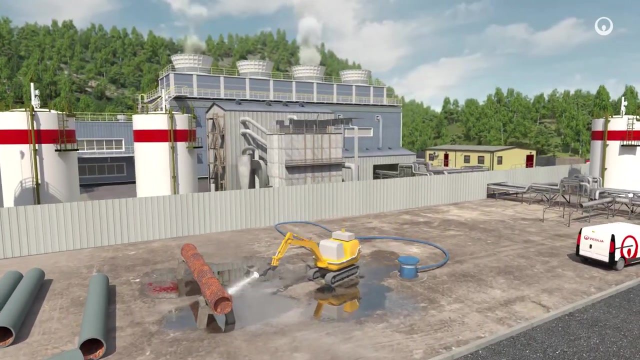 Rich in organic compounds, nitrogen and phosphorus. recycled water helps maintain soil fertility and contributes to reducing the use of chemical fertilizers, promoting more responsible farming practices. Treated water from towns and cities can also be reused by industry: It is used in boilers and cooling towers, for washing plant and equipment or as process water. 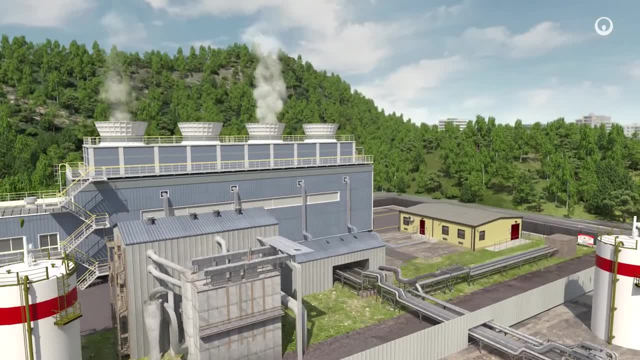 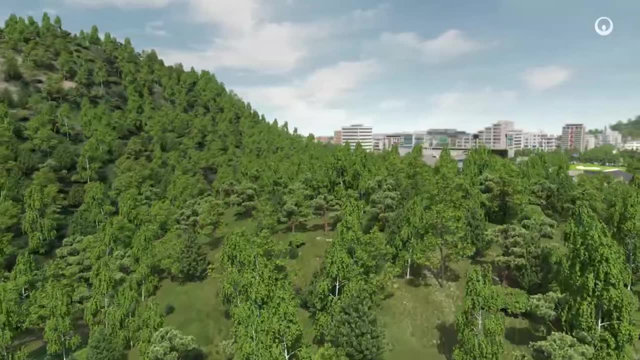 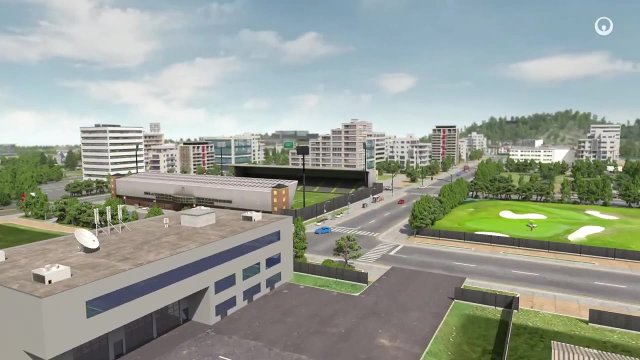 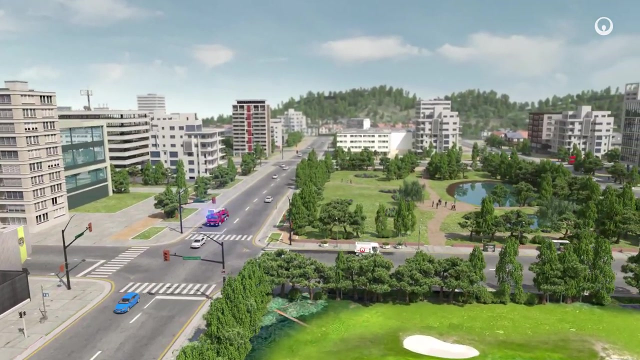 Closed-loop recycling helps industry to move nearer to the goal of zero liquid discharge. Municipalities generally use treated wastewater for purposes where drinking-quality water is not necessary. Recycled water is used for watering sports pitches and golf courses. It can be used for street cleaning, in firefighting systems or for watering parks and open spaces in residential districts. 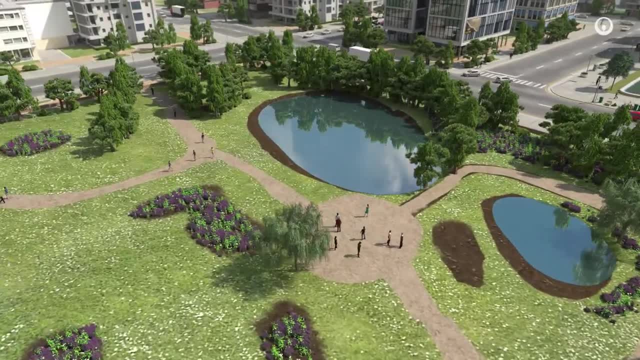 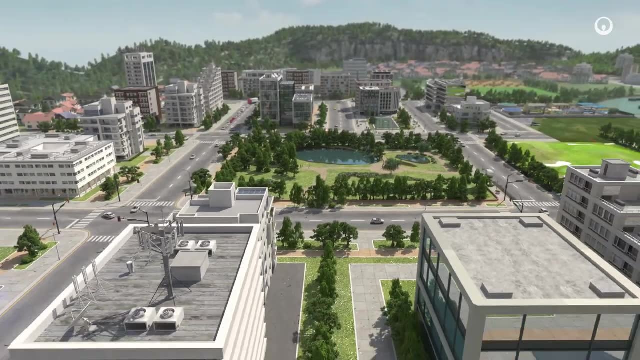 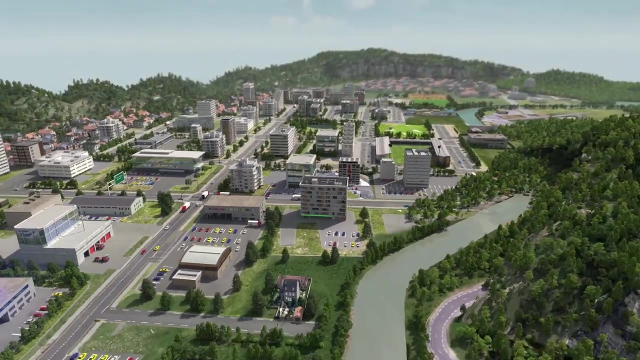 This avoids wasting water resources and improves the quality of life for city residents. Reuse of treated wastewater is one solution for securing access to water. By reducing the impact of water use, this circular economy model protects and replenishes water resources and sustainably extends the water cycle.